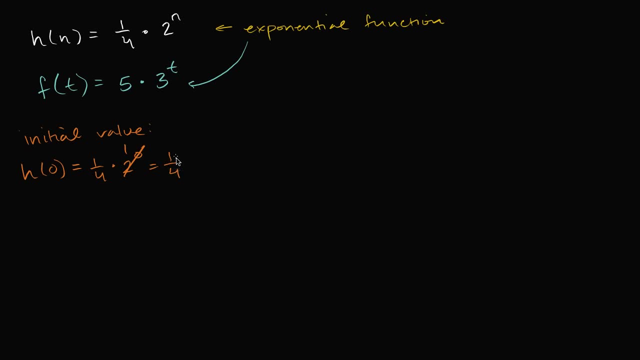 Well, two to the zero, power is just one, So it's equal to 1. fourth So the initial value- at least in this case it seemed to just be that number that sits out here. We have the initial value times some number. 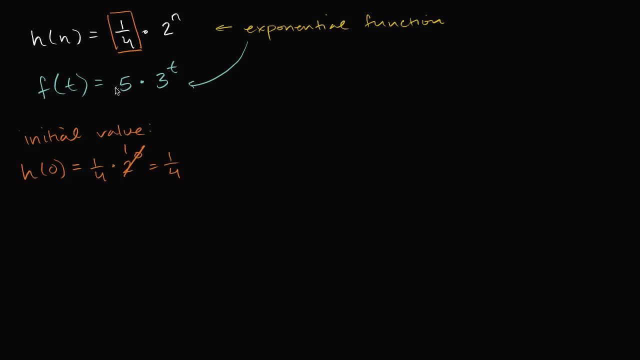 to this exponent And we'll come up with the name for this number as well. But let's see if this was true over here for f of t. So if we look at its initial value, f of zero is going to be five times three to the zero power. 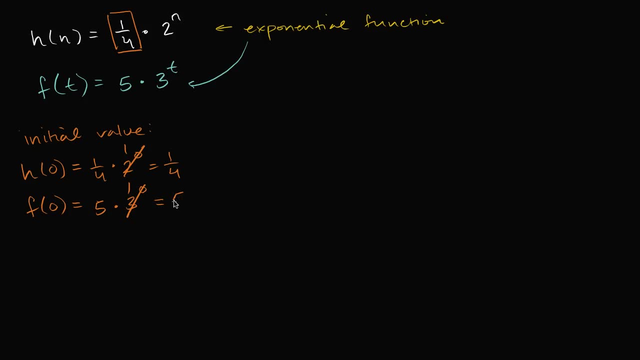 And the same thing again. Three to the zero is just one. Five times one is just five. So the initial value is once again that. So if you have exponential functions of this form, it makes sense Your initial value. well, if you put a zero in for the exponent. 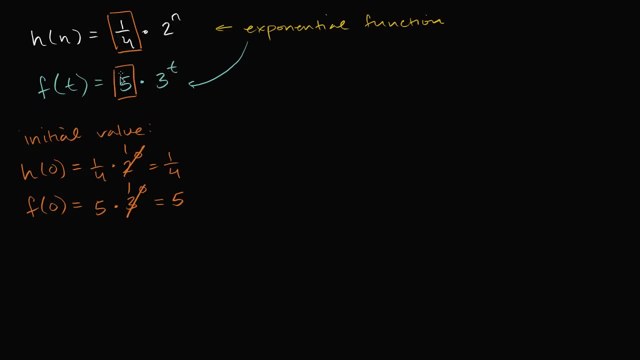 then the number raised to exponent is just going to be one and you're just going to be left with that thing that you're multiplying by that. Hopefully that makes sense. But since you're looking at it, hopefully it does make a little bit. 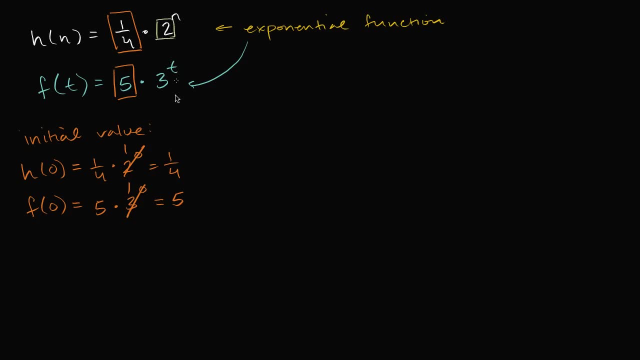 Now you might be saying, well, what do we call this number, What do we call that number there Or that number there? And that's called the common ratio, The common ratio. And in my brain we say, well, why is it called a common ratio? 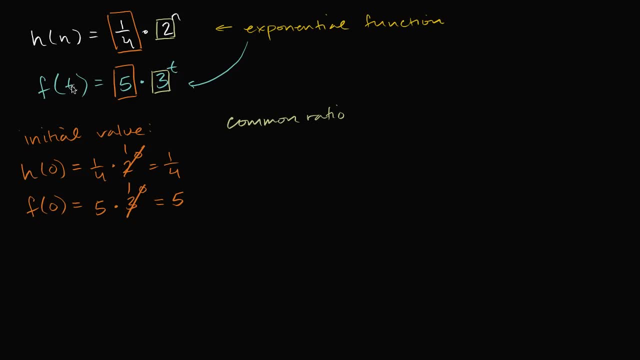 Well, if you thought about integer inputs into this, especially sequential integer inputs into it, you would see a pattern, For example, h of- let me do this in that green color- h of zero is equal to- we already established 1, 4th. 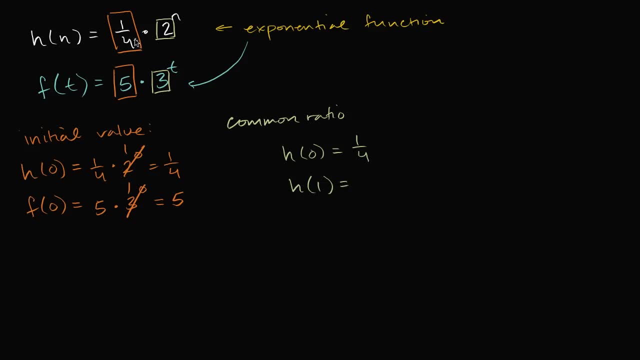 Now what is h of one going to be equal to? It's going to be 1 4th times two to the first power. So it's going to be 1, 4th times two. What is h of two going to be equal to? 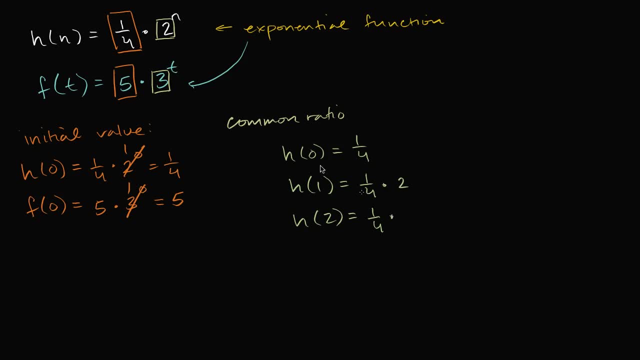 Well, it's going to be 1, 4th times two squared, So it's going to be times two times two, Or we could just view this as this is going to be two times h of one, And actually I should have done this. 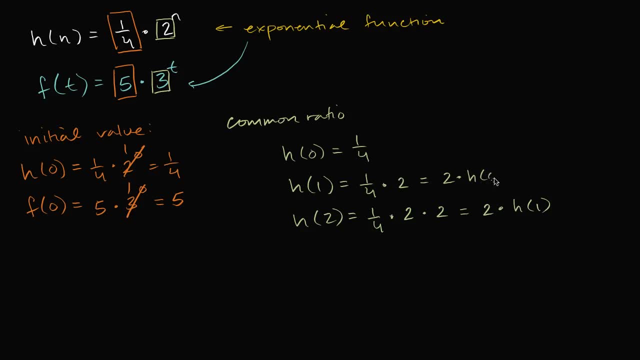 when I wrote this one out. but this we could write as two times h of zero. So notice: if we were to take the ratio between h of two and h of one, it would be two If we were to take the ratio between h of one and h of zero.